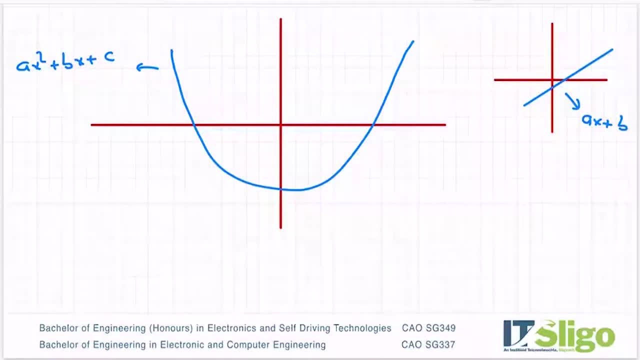 for this one, ax plus b- okay, is a linear function. We have exponential functions, we have cubic functions, we have, and so on and so forth. okay, So there's loads of them. So why are these functions okay? 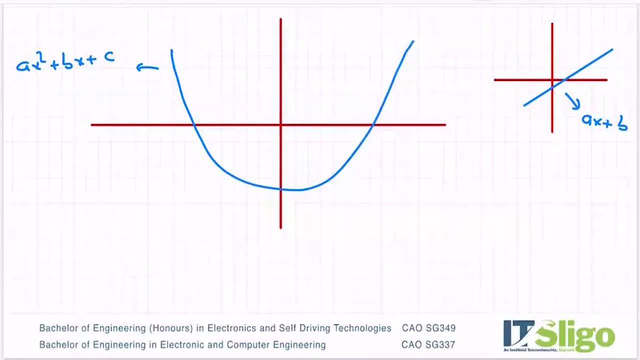 Well, you can do what's called a vertical line test to prove that these are functions okay. And when you do a vertical line test, and a vertical line test means that you draw a vertical line up through your function and if that vertical line that you draw intersects, 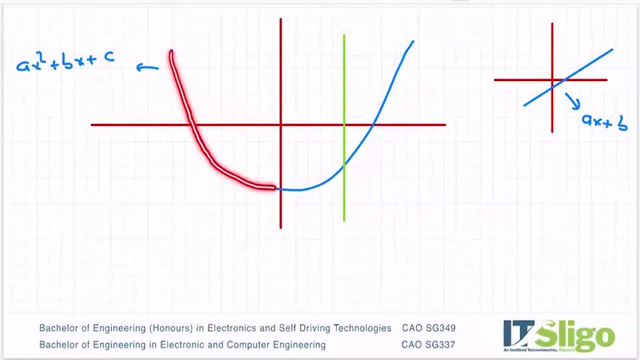 your graph or your function, at most once- okay, Now remember, hear what I'm saying- at most once, then that graph represents a function okay, Or is a function okay, And you should be able to draw that line anywhere. 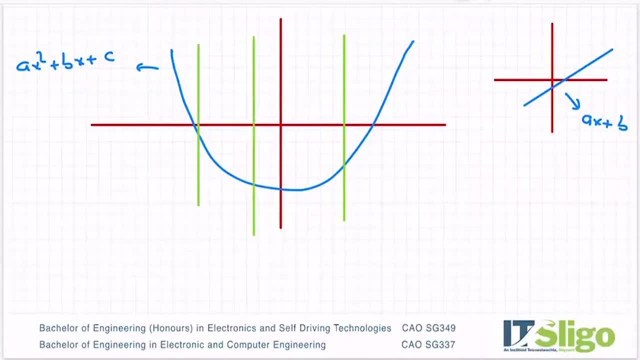 along that x-axis. so for any input, this is our input axis, our x values okay, And our y's are our output values. okay, And that's always the case in functions- any part of the functions chapter okay. 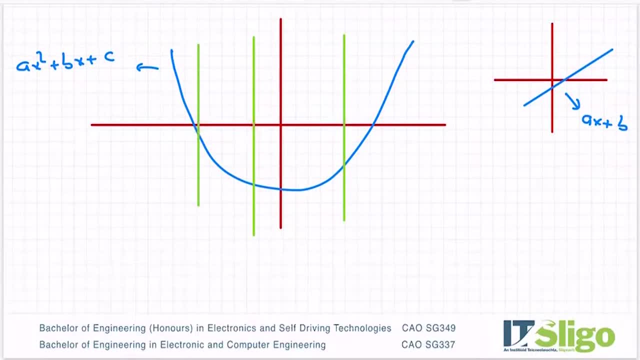 So for any input x I can draw a vertical line and it only intersects the graph at most once. then we consider that a function. okay, And you can see on a line only intersects at most once, okay. So then you might ask me: well, what is not a function? 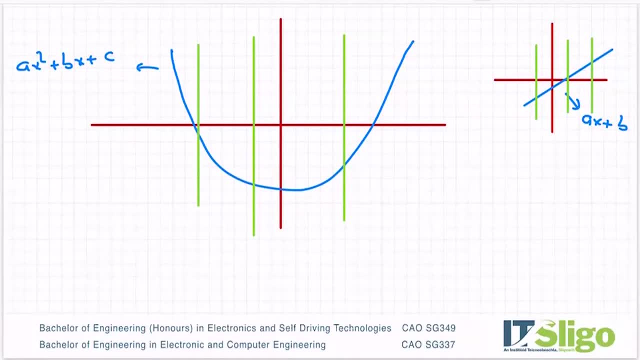 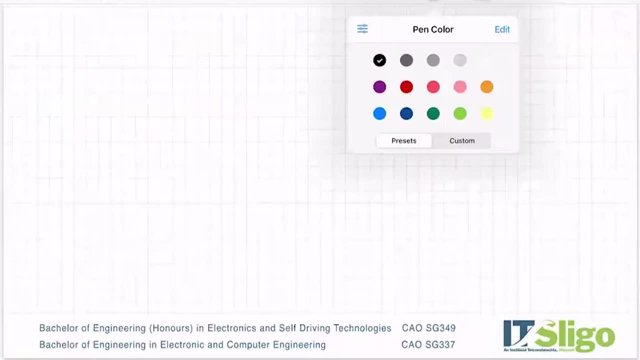 okay, or what does something that? yeah, what does it look like when you don't have a function? okay, So let me again draw in some graphs. So this is what is called a function. We see a different function, okay. 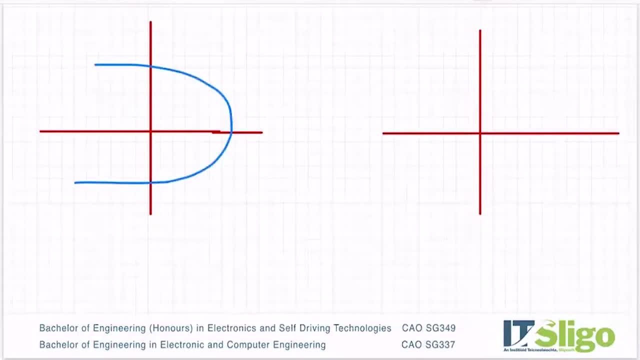 This is the function that we think of as a function. okay, And you show that it's not a function useless. okay, because we're going to write a function if we're not going to use it. So you can see that it's not a function, okay. 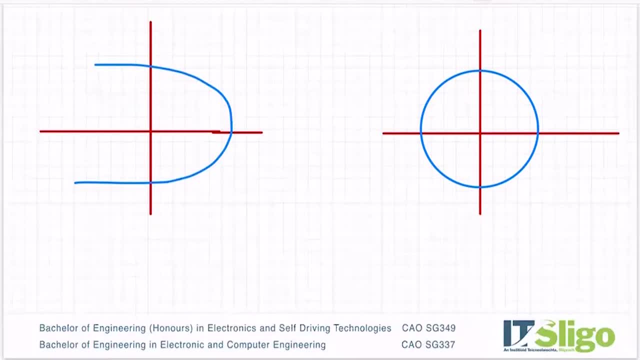 It's a function that works the same way that a function just works the same way that a function works, All right. so let's go back here and I'm gonna show you something else now using the vertical line test. So you take a value of x. 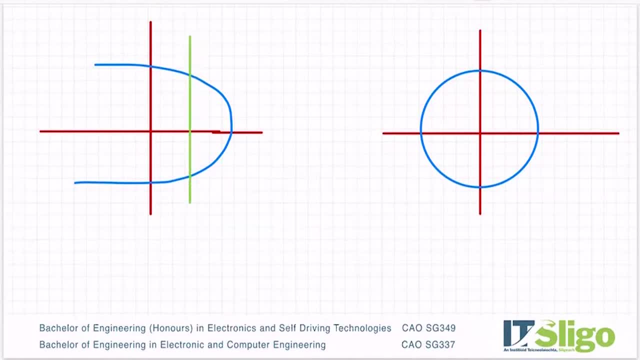 and you show that it fails the vertical line test. okay, It should only intersect the graph at most once. It intersects here and it intersects here, okay. So because it intersects more than once, it is not considered a function. okay, And it's the same for a circle. 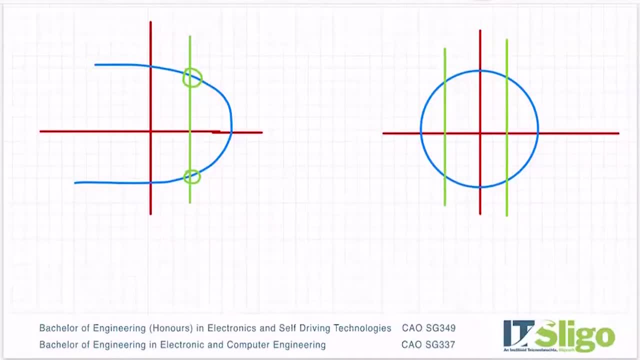 Again, there are values along that where it fails the vertical line test. So therefore, is considered not a function. okay, And in an exam, in a test where you were examining this type of question, if I were to examine it, I would draw a graph something like this: 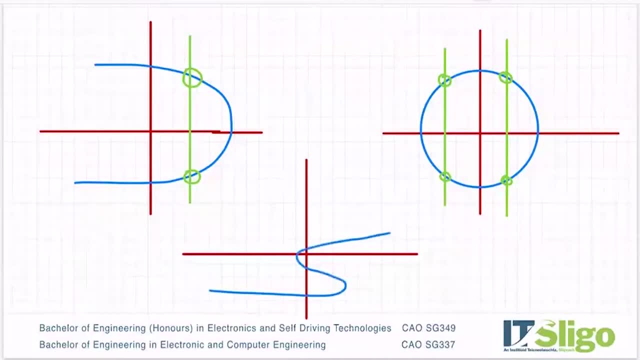 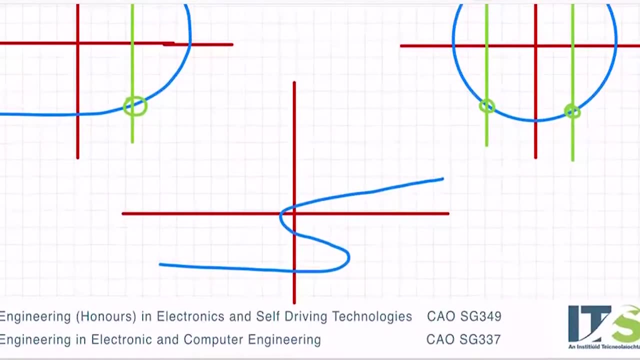 Okay, sorry, I used the line Okay and I would ask you: is that a function And, if not, under what values? is it not a function? okay? Or I would ask you to limit the domain where it could be considered a function. 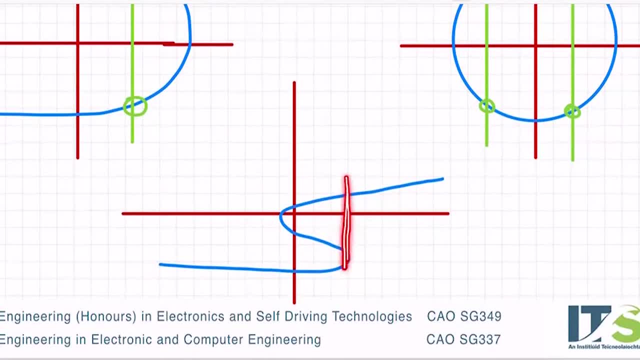 So, in other words, what am I asking there? Well, between this value and this value, it fails the vertical line test. Okay, but if you could limit your inputs or your domain to be any value greater than this number or any value less than this number here, 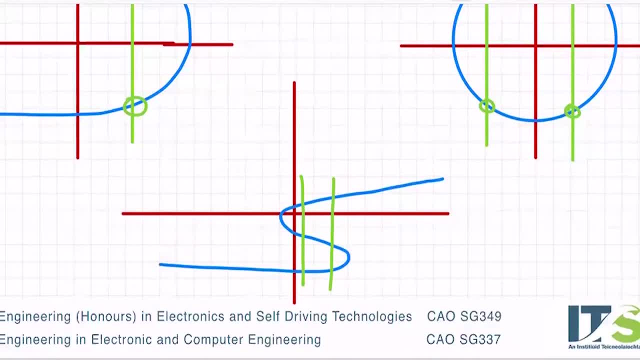 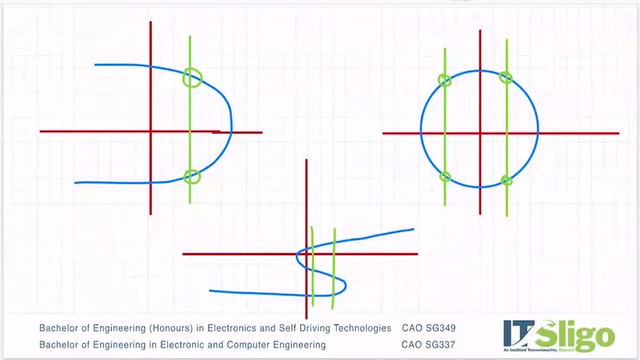 then it wouldn't fail. the vertical line test: okay, I don't think you'd get asked something like that, but you are sometimes asked: under what conditions could a function be called something else? So, in other words, you'll see much more of this. 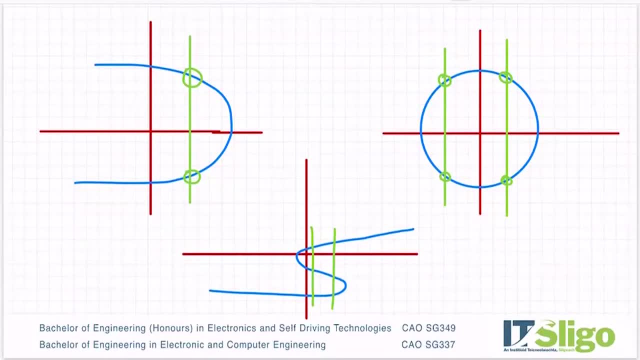 in injective surjective bijective. when we go on to types of functions, You might be asked: under what conditions is the function injective, for example? okay? So all I'm saying here is: see that it's only between these two values. 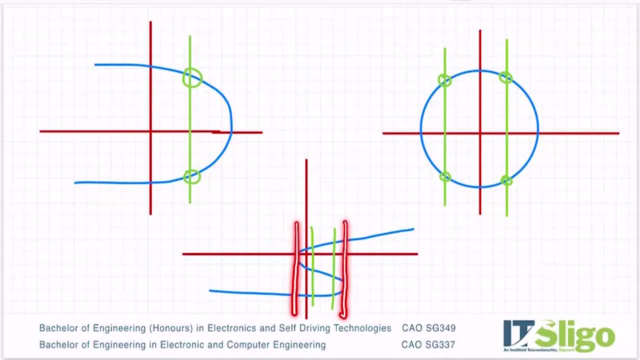 that it fails the vertical line test. okay. So if you have values on your x-axis, you can say: between this and this, it fails the vertical line test, OK. so they are examples of function or examples of, I suppose, graphs that are not functions. 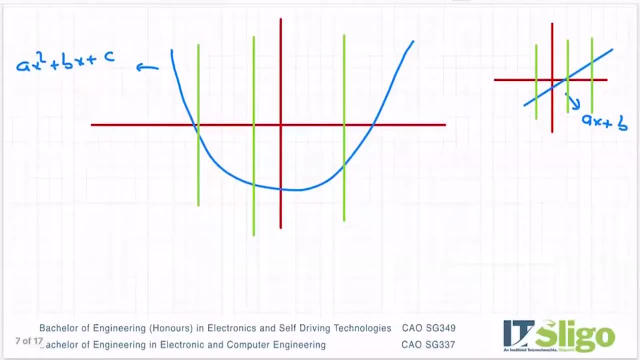 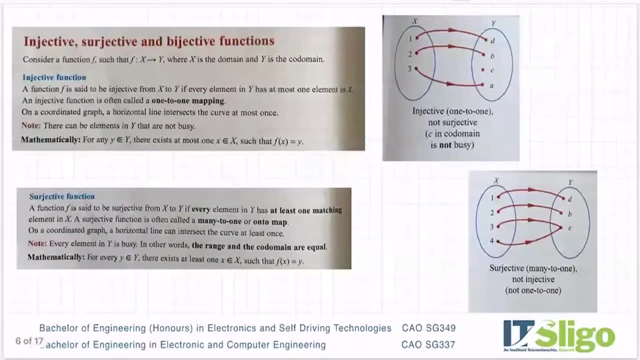 OK. so once you have established that it is a function using the vertical line test, you may then be asked: well, what type of function is it? And the answer to that is either injective, surjective, bijective, OK, or is it one of these? 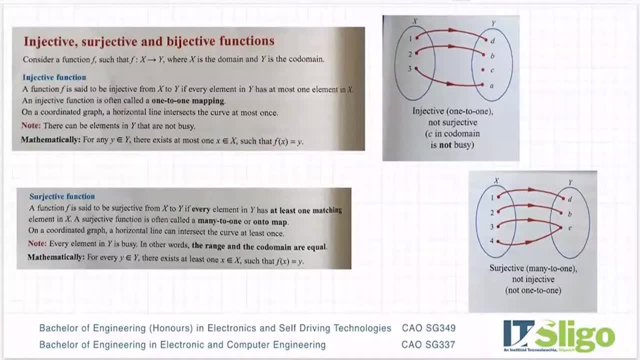 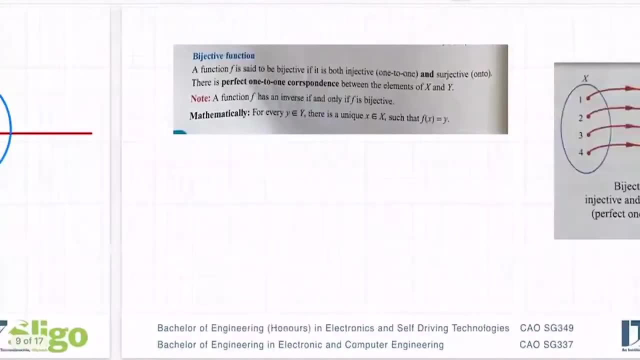 OK, these are the main types and the ones that's on the Leaving Cert course. So I've taken these again from the project maths book, but I also have them from ReviseWise. So I'm just going to go through the two definitions. 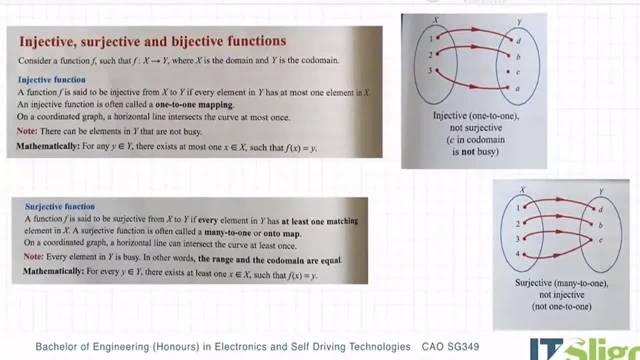 Of all the different types of functions, So injective first. A function f is said to be injective from x to y if every element in y has at most one element in x. OK, an injective function is often called a one to one mapping. 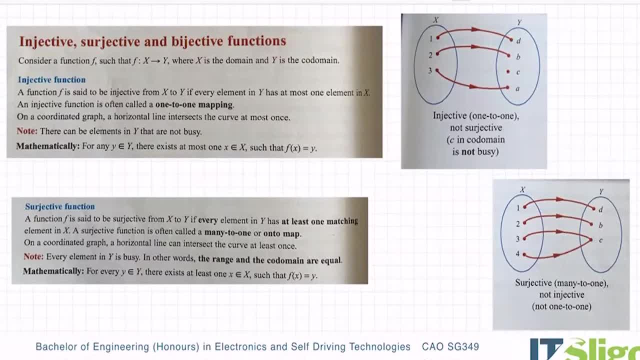 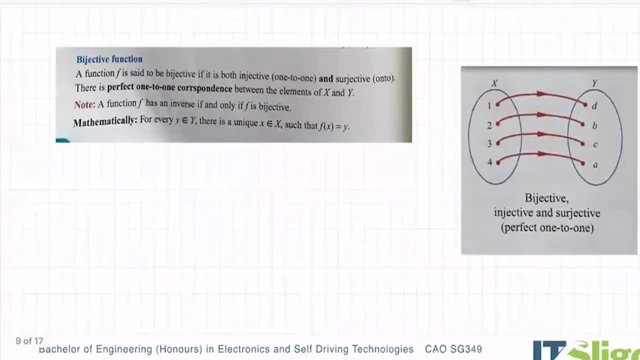 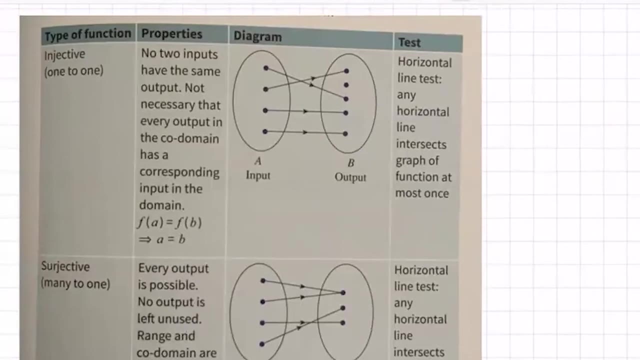 OK. so If every element in y Has at most one element in x, OK, bear with me for a second While I go on to ReviseWise, Because one of these definitions will make more sense in your head and it's different for every person. 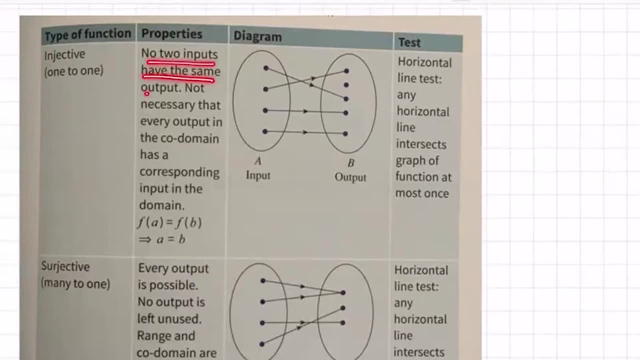 So injective: No two inputs have the same output. No, two inputs have the same output. OK, Not necessary that every output In the co-domain has a corresponding input in the domain. OK, so it's not essential that every output has an input. 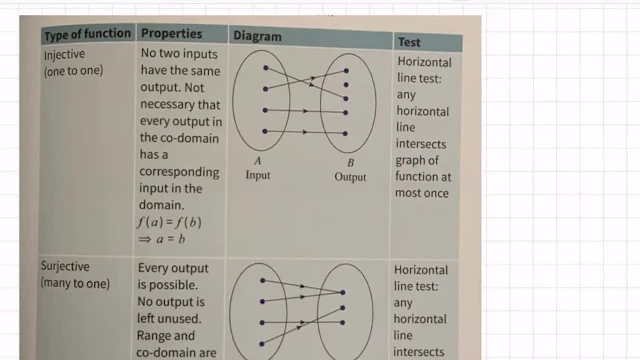 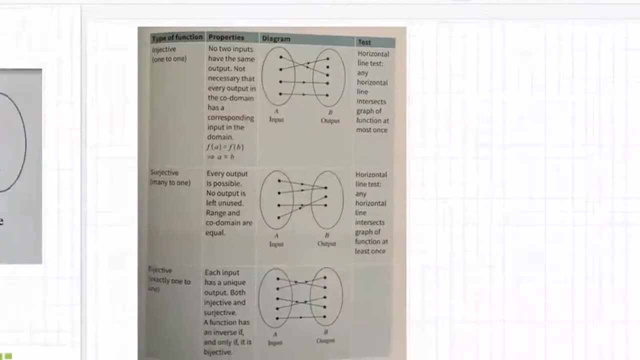 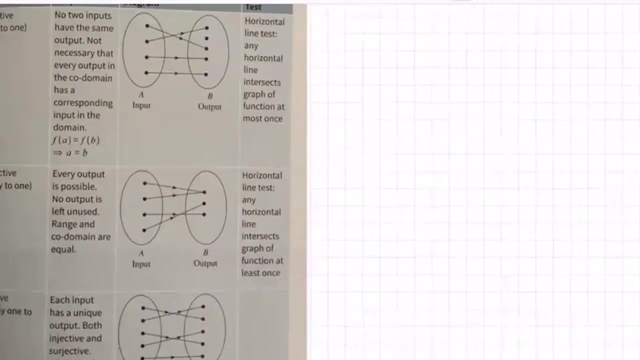 What's important, though, is that no two inputs have the same output. OK, that is an injective function. OK, how do we do? How do we show that something? it's actually written there. How do we show that something is injective? 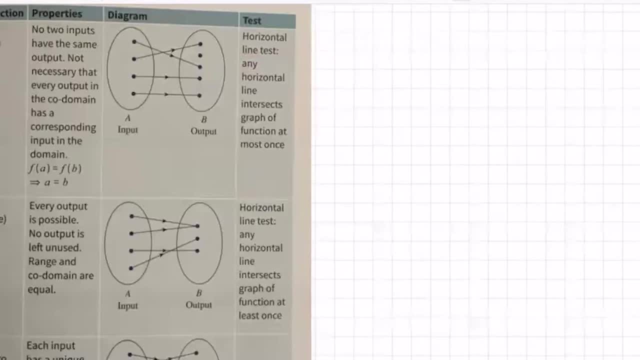 You do a horizontal Horizontal line test and you show that it intersects the graph of the function at most once. OK, so again, let's draw one or two of these and see if we can wrap our head around it. OK, so let's start with our quadratic again. 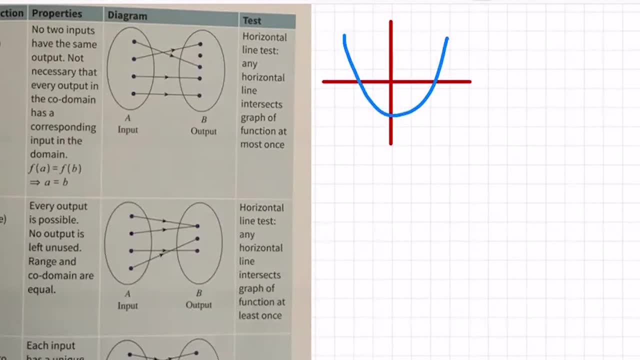 OK, a horizontal line test. OK, so remember, the vertical one is to prove that it's a function. The horizontal one is to test what type of function is it. OK, so Horizontal. Let me draw a horizontal line through this function. 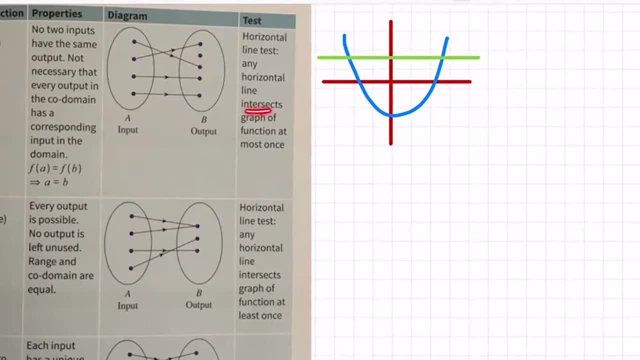 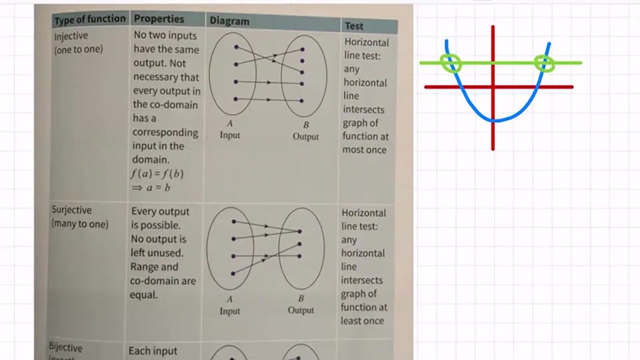 OK, so the horizontal line test intersects the graph of the function at most once. So straight away you can see that this is not an injective function, Because it has intersected the graph at that, you know, at those two X values, whatever they are. 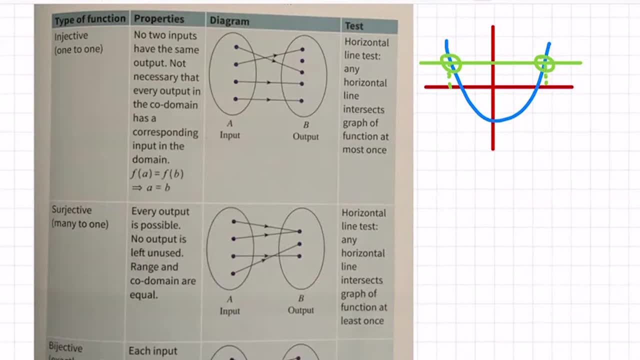 Twice. OK, so an example of An injective function would be a straight line, for example. OK, let me draw that for you. So if I drew into this straight line, then no matter where I draw my horizontal Line test, I am going to intersect that graph. 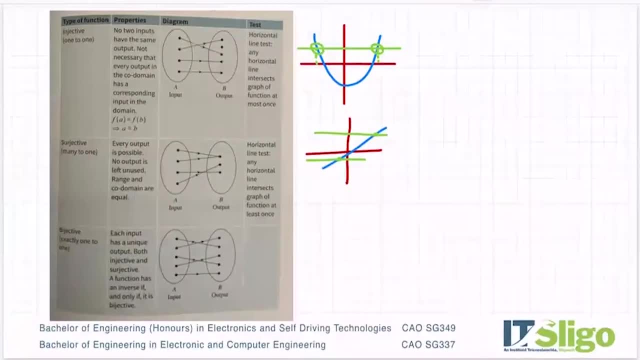 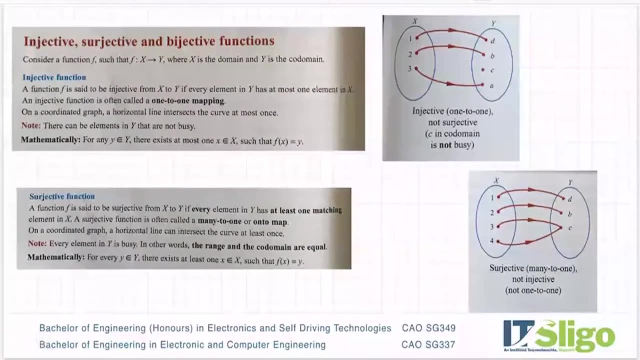 At most once. OK, so that is an injective function. OK, surjective, then A function F is said to be surjective from X to Y If every element in Y has at least one matching element in X. A surjective function is often called a many to one or onto map. 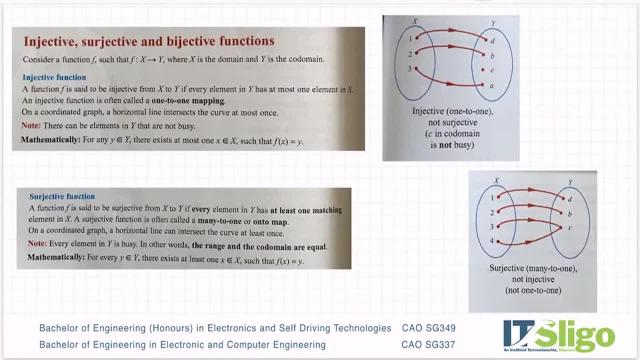 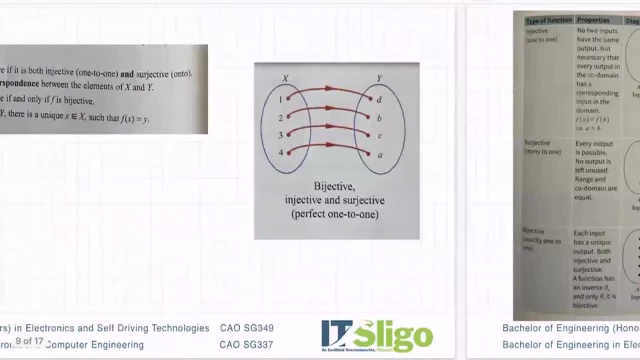 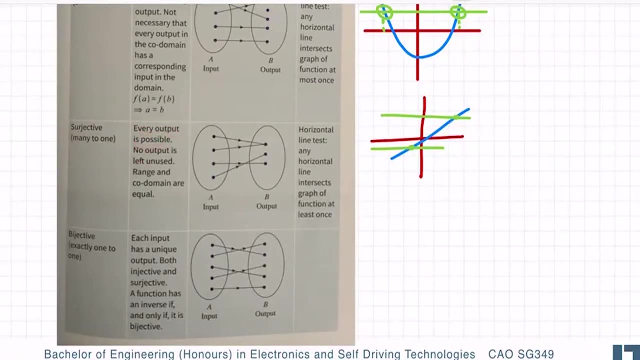 On a coordinated graph, a horizontal line can intersect the curve, At least once. OK. So let's have a look at the other definition: Surjective: Every output is possible. No output is left unused. The range and the codomain are equal. 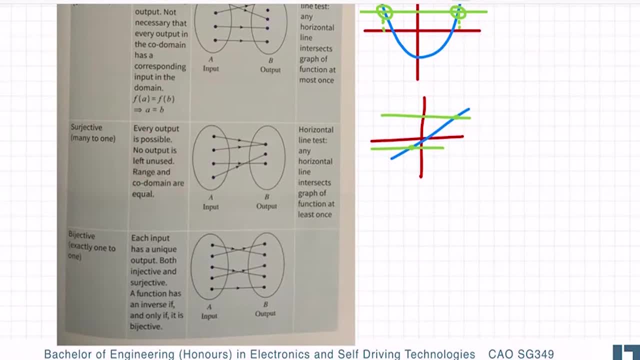 OK, Wait for me for one sec now And I'm going to give you, I am going to give you the, the, the definitions, if I have them here. Yes, so the domain Is the set of input values. OK, so your domain is your input values. 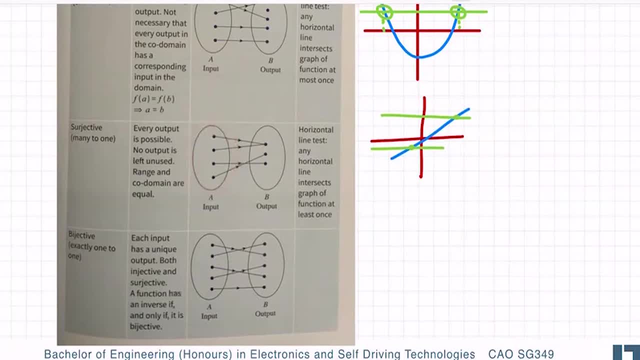 Would be there. in a function, Your range Is the set of output values, And the one we don't hear about too much is this codomain, And codomain is the set of all possible output values. OK, so if you think about a surjective function, because every possible output 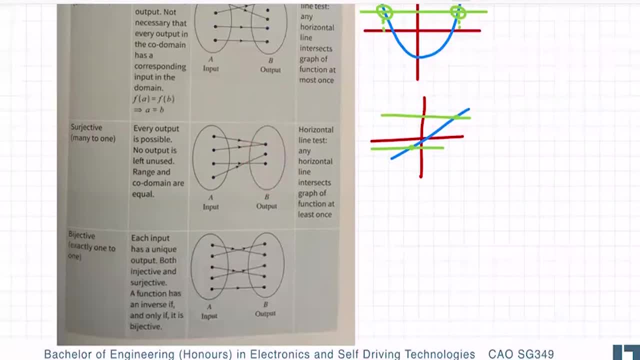 Needs to have an input. OK, every output is possible. Then that is why your range, Which is your outputs, and your codomain, Which is your set of all possible outputs, are equal. OK, so again, I hope that makes sense. 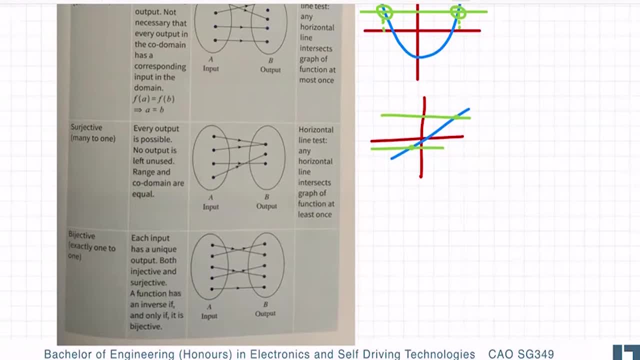 An example of a surjective function is also a straight line, Because if you think about a straight line, it goes on forever. OK, so I could Project this line all the way down and up. These are all my, this is my codomain- all possible outputs. 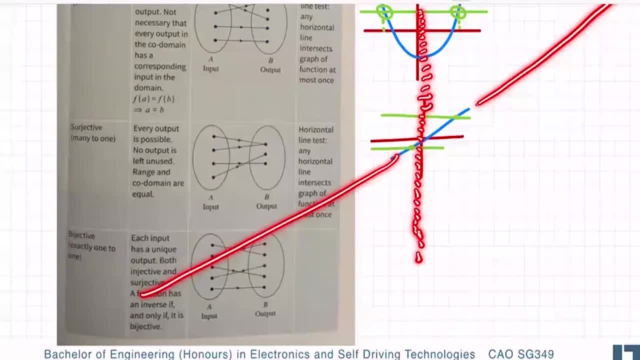 OK, And every possible output. no matter where I do that horizontal line test, I will hit my line graph OK. you can also have other cases where, for example, I'm going to draw an exponential function here now. As such, 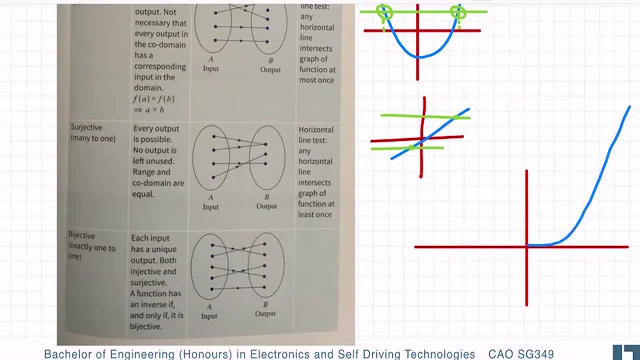 OK, if you limit your range, if you limit your output, OK, and if I said my output, which is Y, was greater than zero, for example, Then my graph could be surjective, OK. so have a look at the range that's specified for that function. 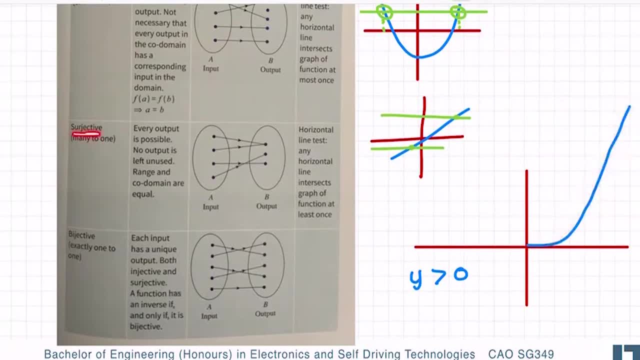 And over that specific range, your function might be surjective OK, so this line could go on like such. So therefore, as long as my outputs are positive, I will have The graph will be surjective. OK, it will pass the horizontal line test. 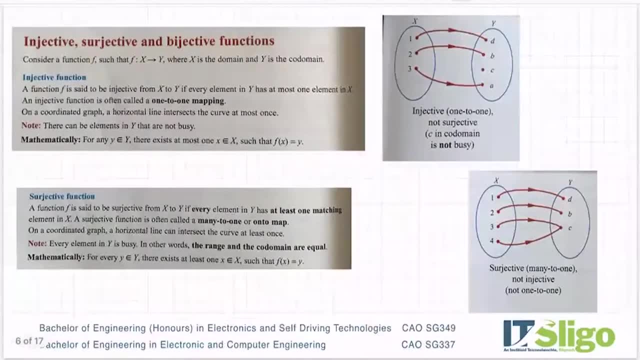 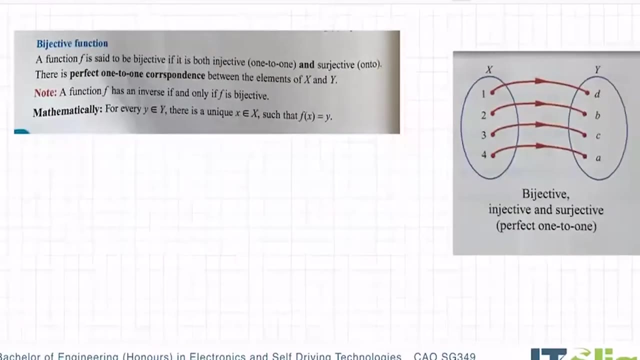 So that's surjective. It might just be surjective over part of the range, It might not be for every real number. So that's injective and surjective. Now, the last one, then, is bijective, And a function is said to be bijective if it is both. 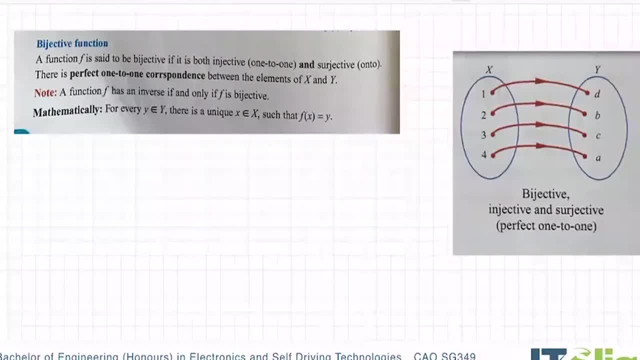 Injective and surjective. So it's the perfect one to one correspondence between the elements of X and the elements of Y. So remember what injective was: Every input had at most one output. Remember what surjective was: Every output had an input. 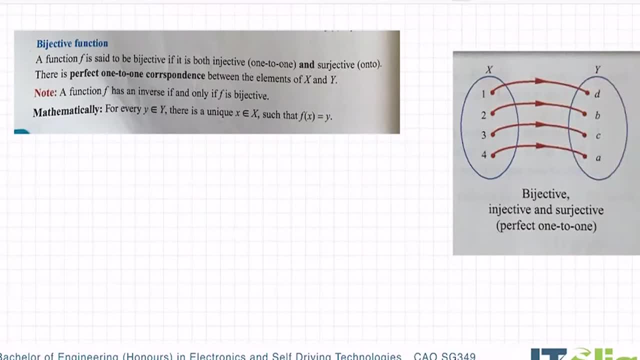 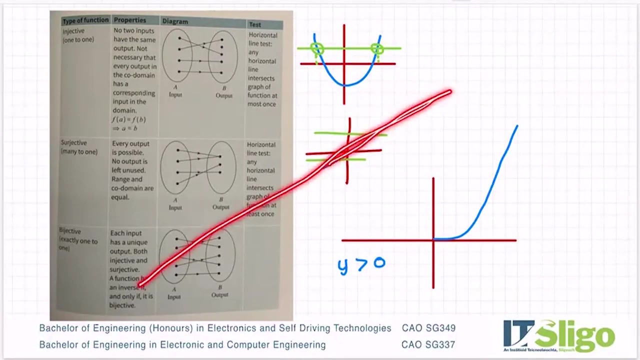 OK, so bijective, It is both injective and surjective, So it's the perfect one to one. And the perfect example of a bijective function is, of course, the line OK, because that is both injective and surjective. 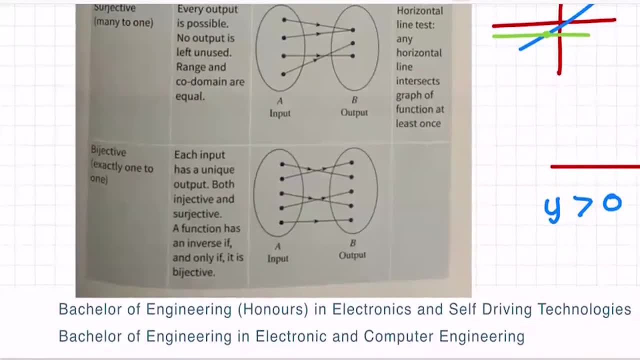 And it's why I used it for the, for the example, for both. So then the revise wise description. each input has a unique output, both injective and surjective. OK, a function has an inverse if, and only if, it is bijective. 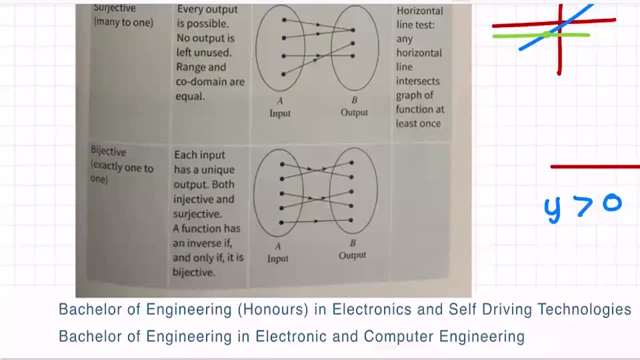 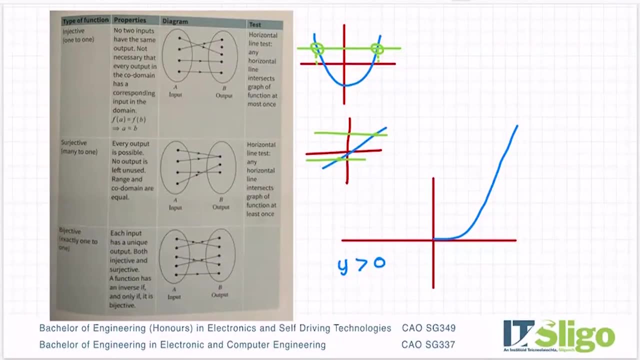 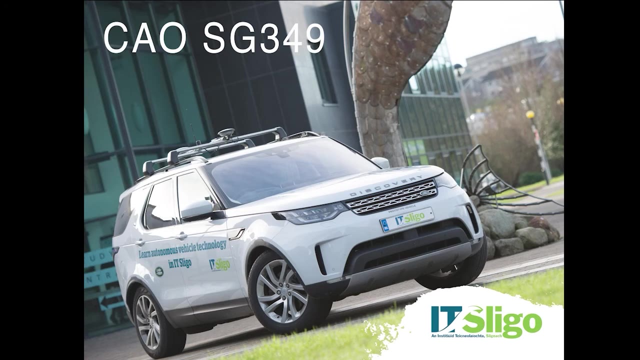 OK, and I'll come back to that in a few minutes- when we look at inverse functions. So that is bijective. So to show something is bijective. you're showing that it's both injective and surjective. first, If you've enjoyed this video, then why not join us in IT Sligo and use maths in practice? 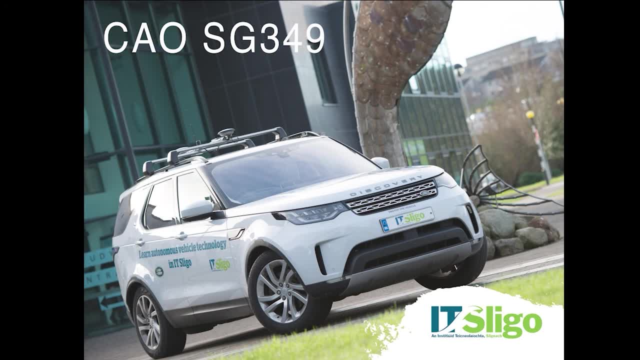 In conjunction with industry, we've designed an exciting new program in electronics and self-driving technologies which uses cutting edge techniques such as artificial intelligence, computer vision and virtual and augmented reality. You'll need a H5 in maths to qualify. Check out the link below.